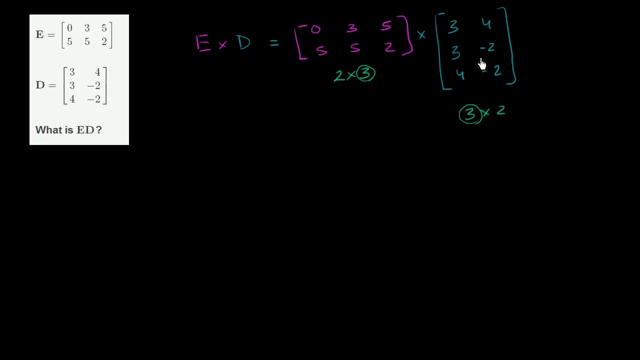 if the number of columns here were not equal to the number of rows here, then this would not be a valid operation, at least the way that we have defined matrix multiplication. The other thing you always have to remember is that E times D is not always the same thing as D times E Order. 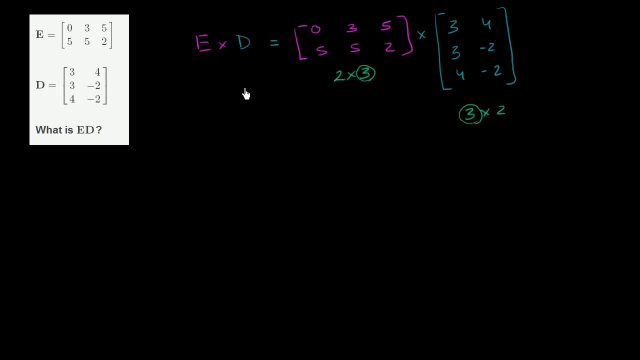 matters when you're multiplying matrices. It doesn't matter if you're multiplying- you're not multiplying regular numbers, but it matters for matrices. But let's actually work this out. So what we're going to get is actually going to be a 2 by 2 matrix. 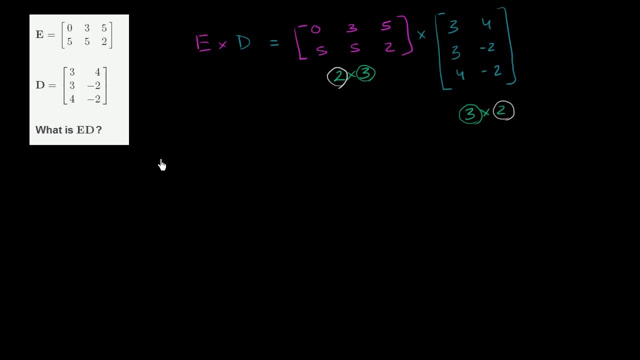 But I'm going to create some space here because we're going to have to do some computation. So this is going to be equal to: I'm going to make a huge 2 by 2 matrix here. So the way we get the top left entry, the top left entry. 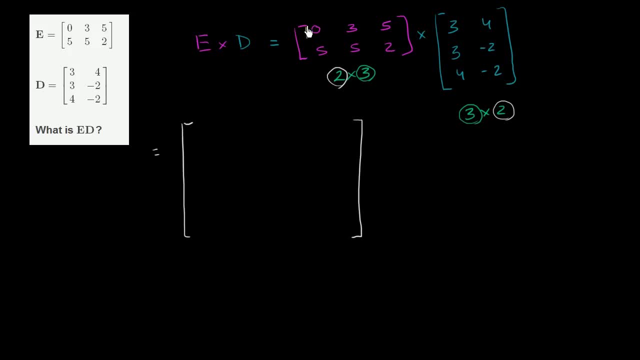 is essentially going to be this row. It's going to be this row, It's going to be this row times this product. If you viewed them each as vectors and you have some familiarity with the dot product, we're essentially going to take the dot product of that and that. 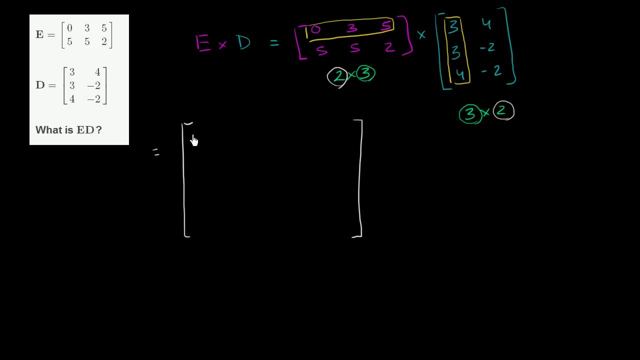 And if you have no idea what that is, I'm about to show you. This entry is going to be 0 times 3 plus 3 times 3 plus 5 times 4.. So that is the top left entry, And I already see that I'm going to run out of space here. 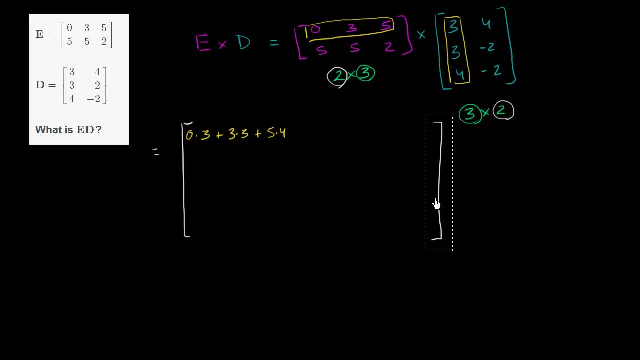 so let me move this over. So let me move this over. Let me move this over to the right. some space, so I have some breathing room. Now we can do the top right entry. This was the top left. Now we're going to do the top right. 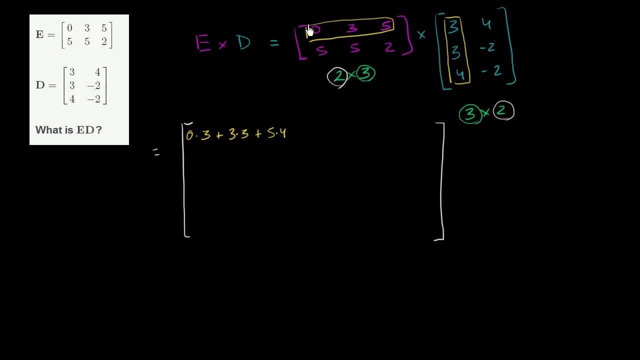 So the top right entry is going to be this: row times this column. Notice, the entry is getting the row from the first matrix and the column from the second one. That's kind of determining its position. So once again, it's going to be 0 times. 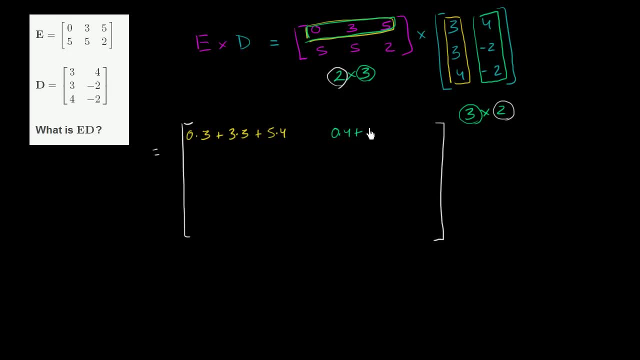 4 plus 3 times negative, 2 plus 5 times negative 2.. And we keep going. The bottom left entry is going to be this row. the second row here times the first column here, So it's 5 times 3 plus 5 times 3 plus 2 times 4..